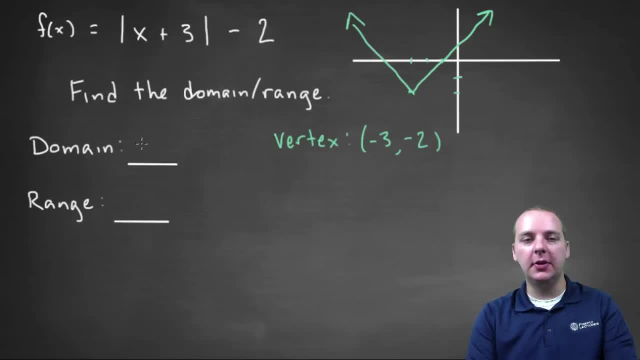 just because it's the absolute value function, the domain is going to be all real numbers. So minus infinity to infinity. Now how did I know that so fast? There's no X that I couldn't take the absolute value of, So this. 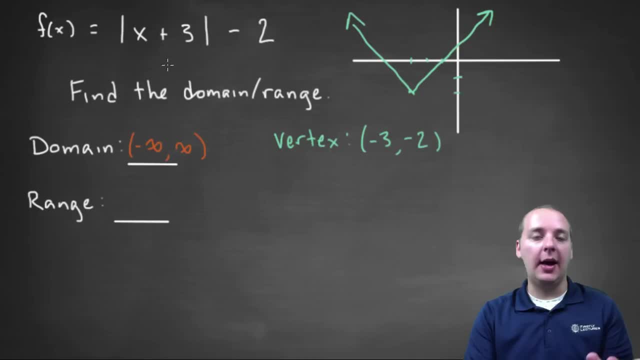 the absolute value function causes no problems. I would never get division by zero, I would never have a negative under a square root, because there's not a square root and there is no division And so if it's just an absolute value type function, the domain will be all. 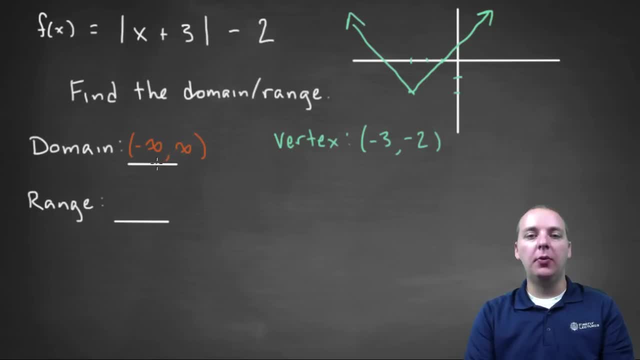 real numbers. Alright, now what about the range, though? Well, the range will be some from some Y value up or some Y value down, depending on if the V shape graph opens upward or downward. Ours opens upward, So ours will be Y greater than or equal to some certain Y value, If 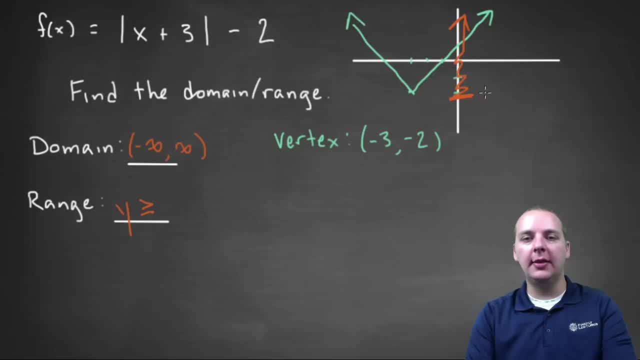 you look at the graph, it looks like it's higher than about this Y value. Now, where is this Y value right here? Well, notice, that's just dictated by the vertex, And so, like I said, even without the graph, you can just think about where the vertex is, in this case negative. 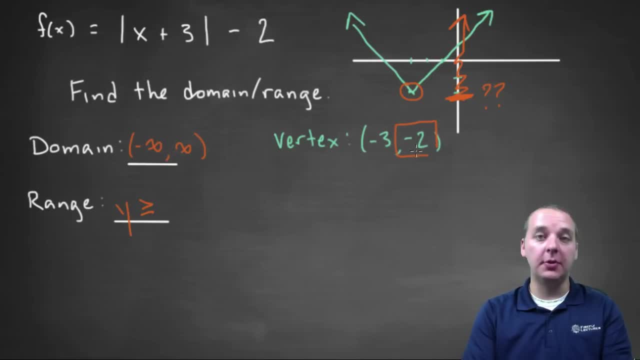 two. negative three comma negative two, but I'm I'm concerned about the Y value, Obviously being that this is the range, And so the range will be all the Y values above or greater than negative two, And so that will be your final answer, So notice. 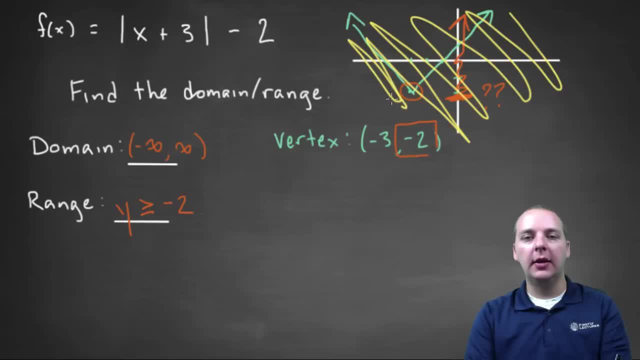 you know, even if we didn't have this graph right here, you know as long as you could look at this function and see where the vertex was then and you knew if the graph opened up or down, then you would just say the domain is all real numbers and the range is Y greater. than or equal to Negative two right here.